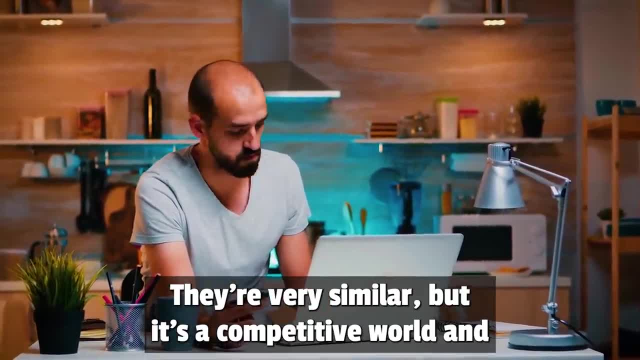 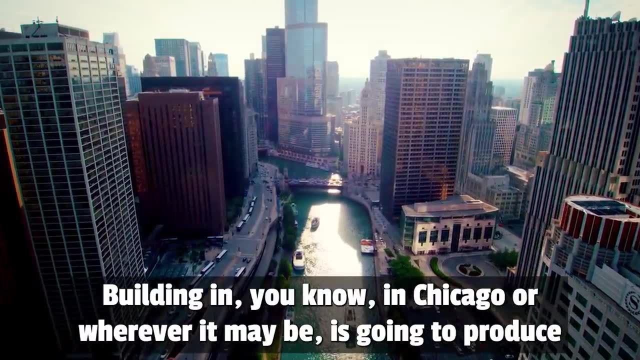 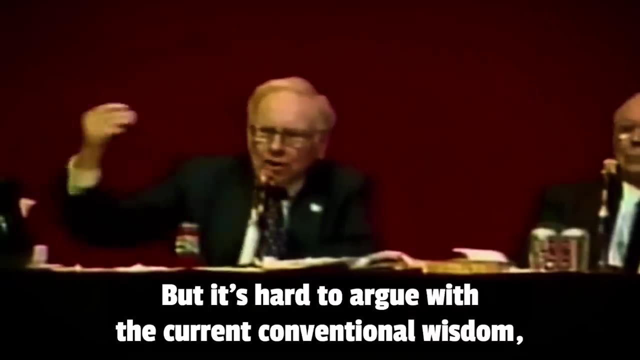 they're very similar. but it's a competitive world and you know, they all know about what a class, A office building, and you know Chicago, or wherever it may be, is going to produce- At least they have. they may all be wrong, as it turns out, because of some unusual events, but but it's hard to argue with the current conventional. 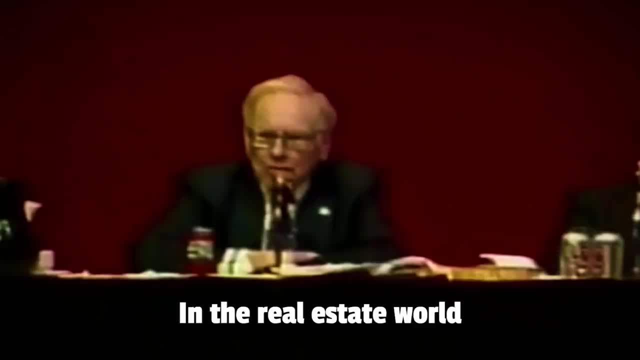 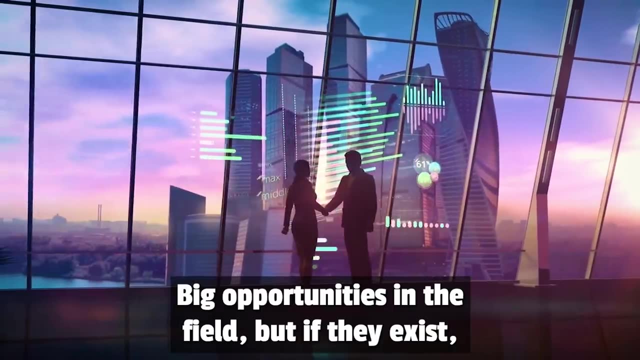 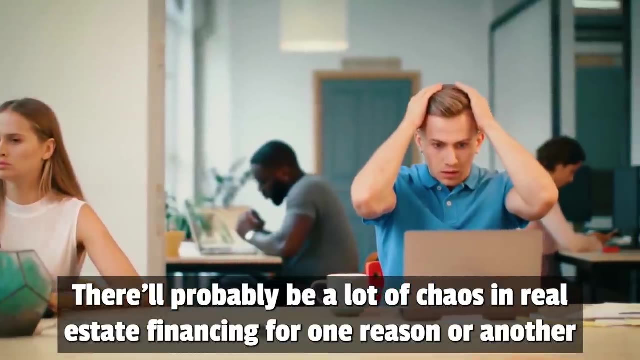 wisdom most of the time in the real estate world, But occasionally there have been some. you know there there could be big opportunities in the field, but if if they exist, it will certainly be because there's a there. probably there'll be a lot of chaos in real estate. 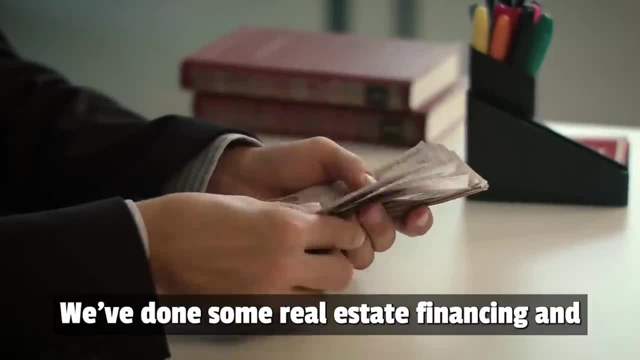 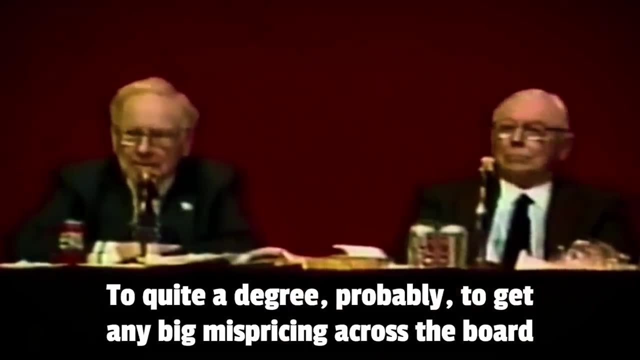 We've done some real estate financing. for one reason or another, We've done some real estate financing and you have to have the money shut off to quite a degree probably to get any big mispricing across the board. Charlie, Yeah, we don't have any competitive advantage. 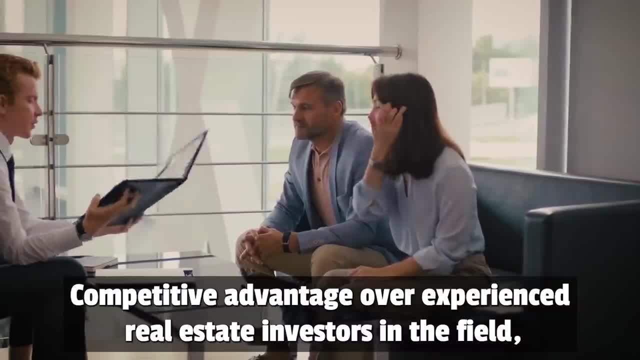 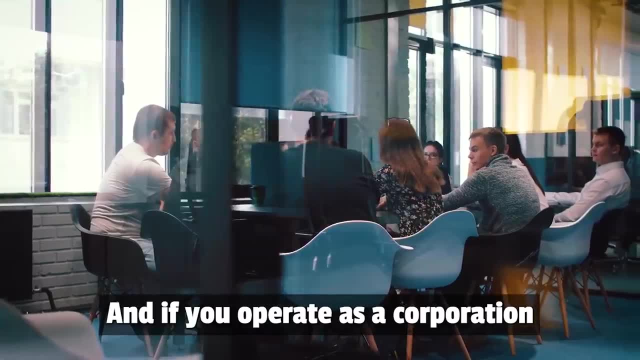 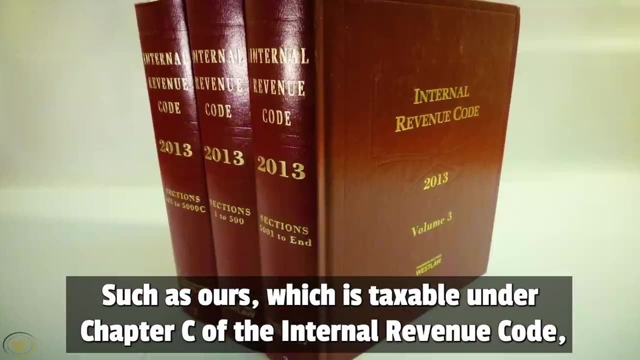 over experienced real estate investors in the field, and we wouldn't have if we were operating with our own money as a partnership. and if you operate as a corporation such as ours, which is taxable under chapter c of the internal revenue code, you've got a whole layer. 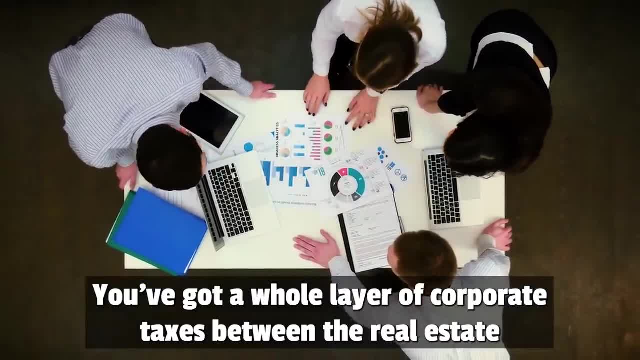 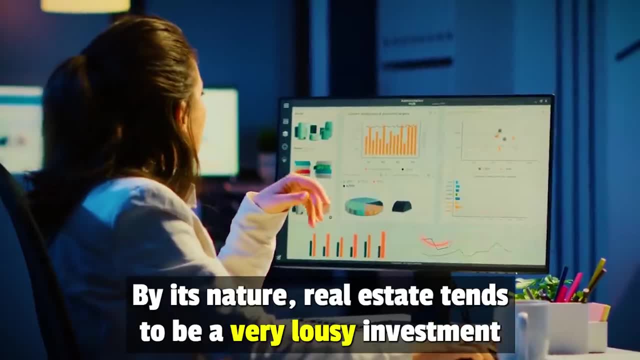 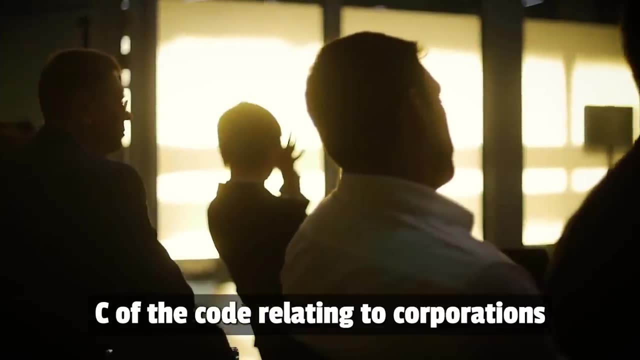 of corporate taxes between the real estate income and the use of the income by the people who own the real estate. So by its nature, real estate tends to be a very lousy investment for people who are taxed under sub chapter c of the code relating to corporations. So the combination of 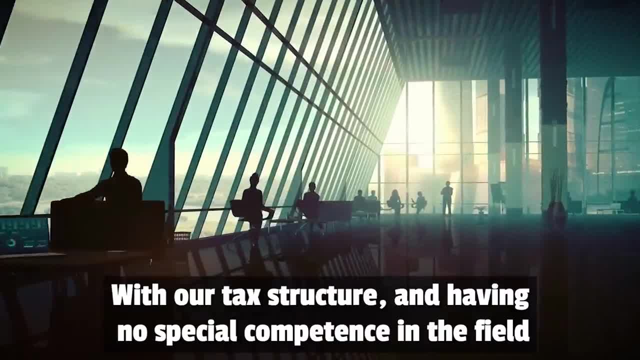 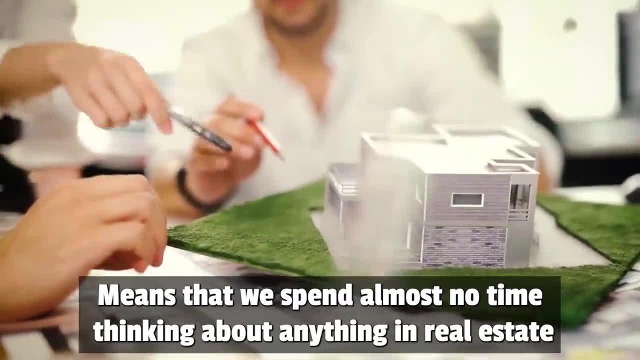 having it generally a lousy activity for people with our tax structure and having no special competence in the field, means that we spend almost no time thinking about anything in real estate, and then such real estate as we've actually done, like holding surplus real estate and trying 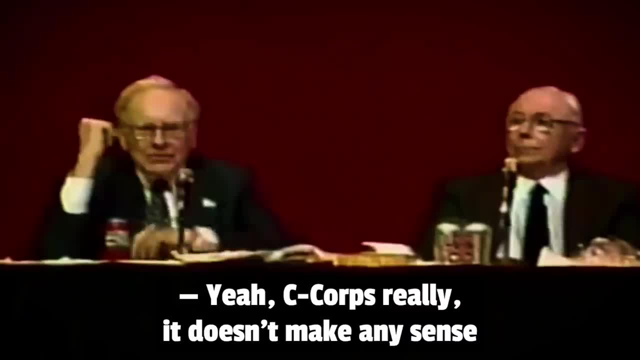 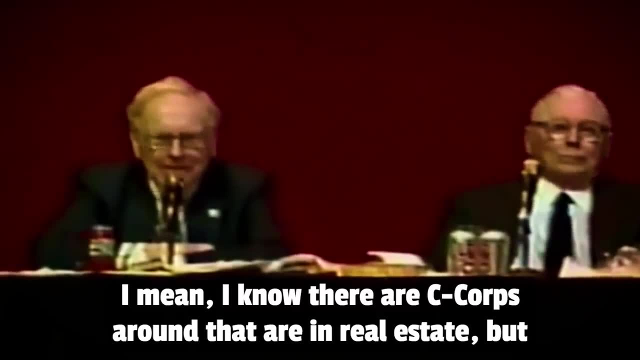 to sell it off. I'd say we have a poor record at, Yeah, c-corps. really it doesn't make any sense. I mean I know there are c-corps around that that are in real estate, but there are other structures more attractive. There really aren't other structures. I mean Lloyd's is an attempt at it.